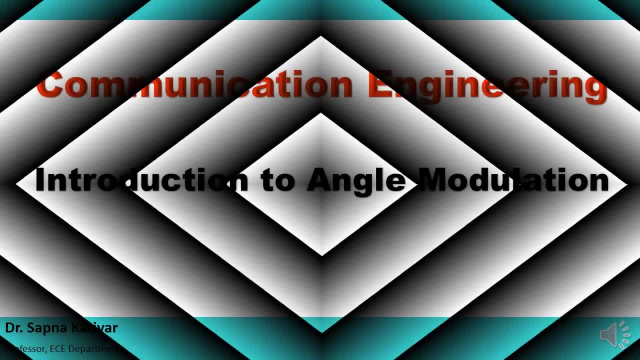 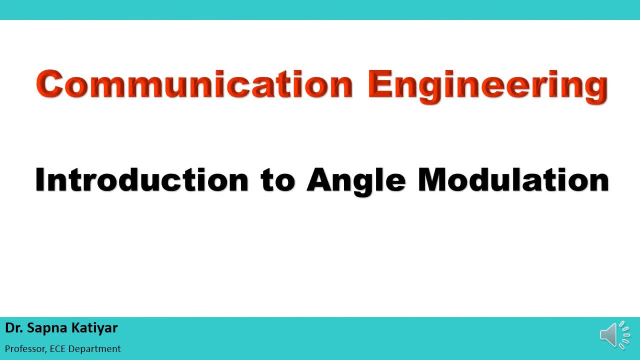 Hello everyone, welcome to video lecture series of communication engineering. Today's topic is angle modulation. Before starting today's video, let me tell you that in previous videos I have discussed about the amplitude modulation, where amplitude of the carrier varied according to the message signal, and we have also calculated the bandwidth of amplitude modulated signal. 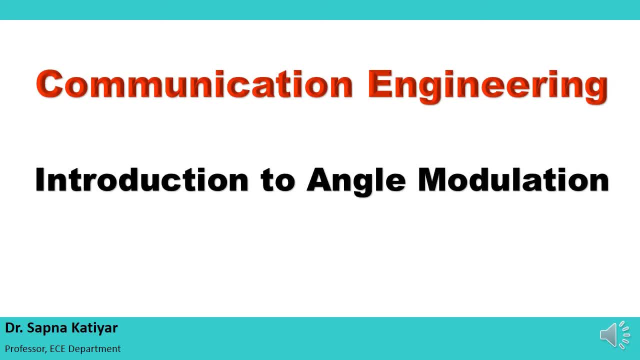 and the bandwidth never exceed twice the maximum frequency component which is present in the AM signal Twice of FM is the maximum bandwidth. So there is another significant method of modulation which is known as a angle modulation. So let us begin Angle modulation. 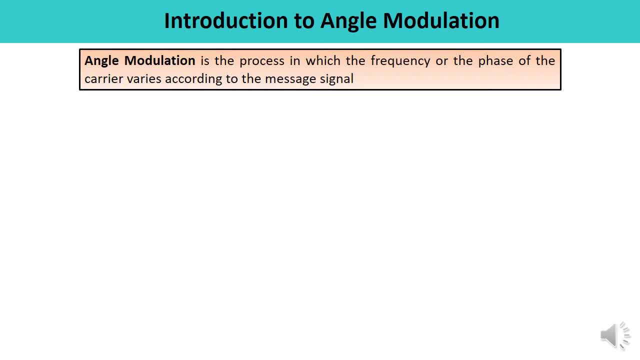 Angle modulation. it is defined as the process in which the total phase angle of a carrier is varied according to the instantaneous value of the modulating signal or message signal, and here the amplitude of carrier is kept constant. So in this particular way you can explain what is. 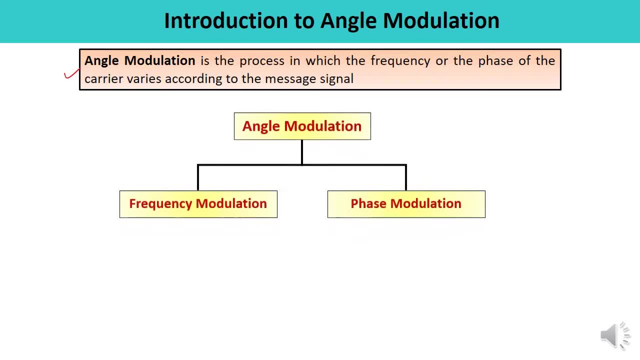 angle modulation. Angle modulation is also of two types. One is called the amplitude modulation and the other is called the amplitude modulation. One is frequency modulation and second is the phase modulation. So frequency modulation as well as phase modulation. they forms the angle modulation. An angle modulation has several. 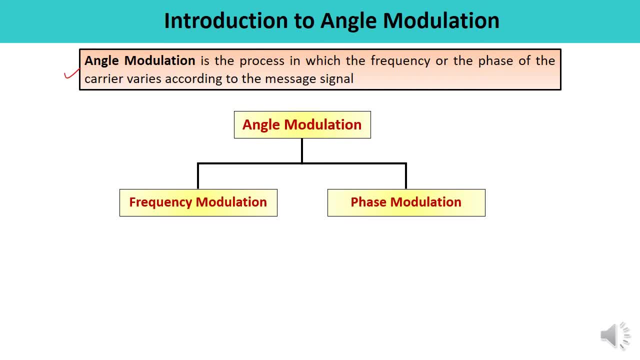 advantages over amplitude modulations. The advantages are like noise reduction, more efficient use of power, but there are few disadvantages. also, Let us talk what is frequency modulation? So in case of the frequency modulation, you can define it as a process of varying frequency of carrier signal linearly with the message signal. 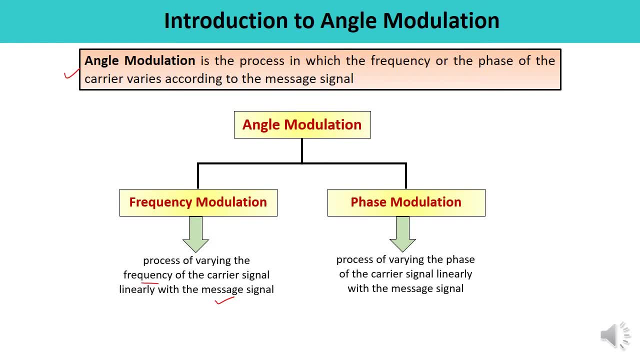 While in case of phase modulation it is a process where the phase of the carrier signal varied according to the message signal. It means if frequency of carrier is varying according to the message signal, the type of modulation is frequency modulation, And if phase of the carrier is varying according to the message signal, then the type of modulation is phase modulation. 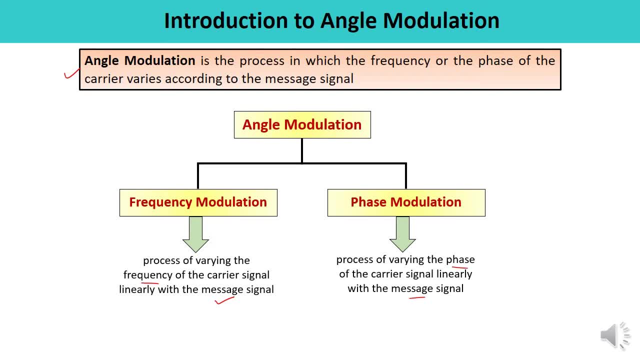 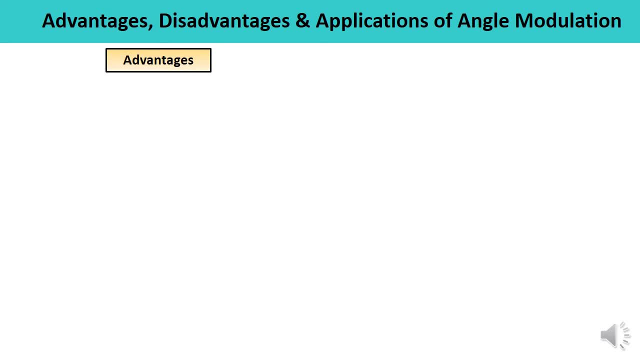 So in coming slides I am going to discuss about these two in detail. Let us discuss advantages, disadvantages and applications of angle modulation. So, just starting with the advantages, as I have already told you that there are various advantages of angle modulation over amplitude modulations. 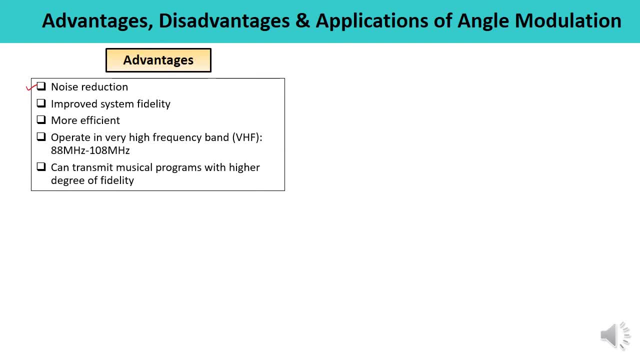 Noise reduction: noise is less improved system fidelity: this system is more efficient. angle modulation: this operates in very high frequency band. it approximately ranges from 88 MHz to 108 MHz and it can transmit musical programs with higher degree of fidelity. 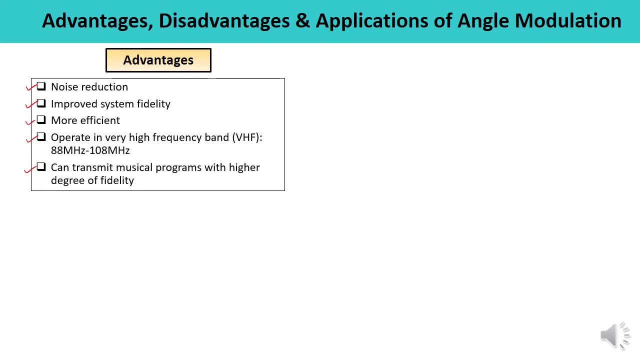 But at the same time there are some disadvantages. also The types of circuits which are used in the case of the angle modulation. They are quite complex and bandwidth is also increased in this particular case. So these two are the major disadvantages. There are various applications of the angle modulation. 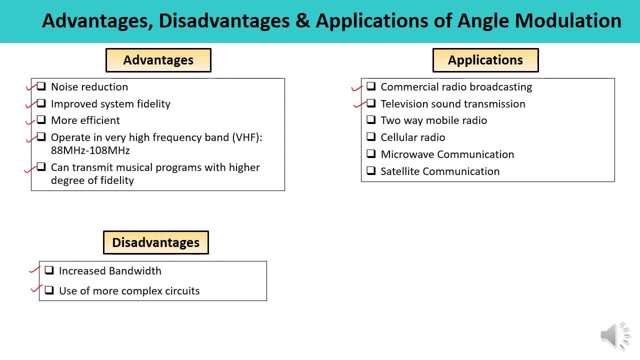 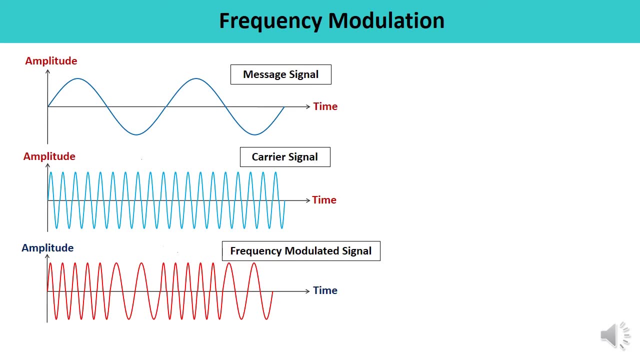 It can be successfully employed for radio broadcasting, for television, sound transmission, Two way: mobile radio, cellular radio, microwave communication, satellite communication. So there are various applications of the angle modulation. First let us discuss about the frequency modulation. What is frequency modulation? 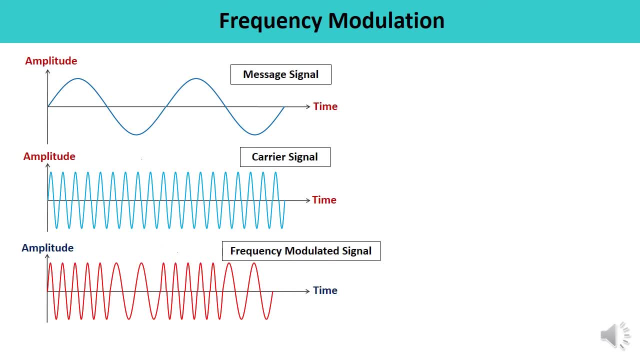 We have understand, the frequency modulation is a process where carrier frequency of the carrier is varied according to the message signal. You can see in this particular diagram: first is the message signal, second is the carrier signal is being shown And the third is the frequency modulated signal is being drawn over here. 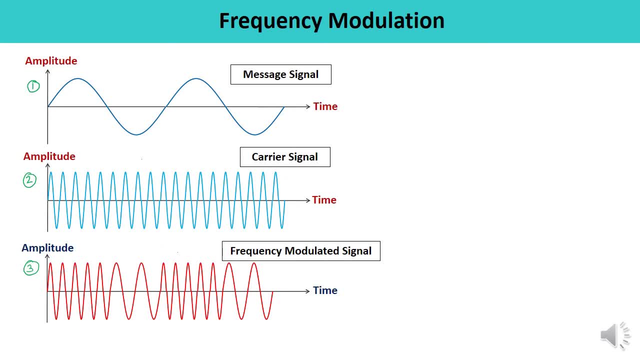 Here you can see: carrier signal is varied according to the message signal. So when the message signal is frequency, this amplitude is increasing Means. you can see over here in this particular case, in the case of the message signal during the positive half cycle. 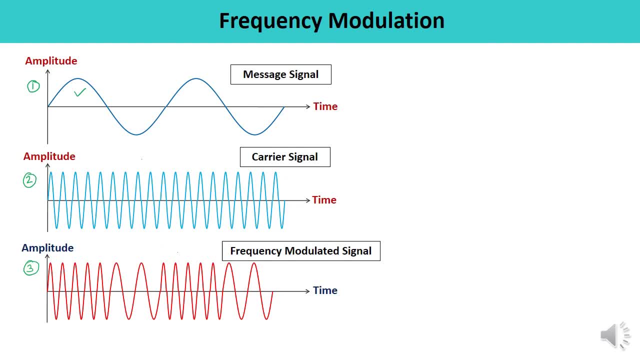 when the amplitude increases, the frequency also increases, and the same you can observe in this particular diagram During the negative half cycle. you can observe over here: when the amplitude decreases, the frequency also decreases, and the same pattern you can observe over here. 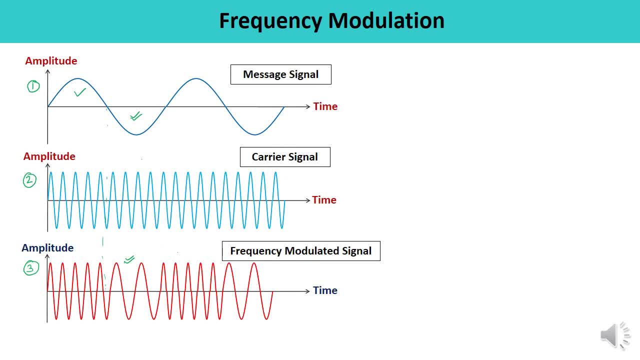 Again during the positive half cycle, frequency increases, then decreases. So the frequency varies according to the carrier signal. This is what we have discussed over here. It means you can define frequency modulation. It is a type of angle modulation. So this is what we have discussed over here. 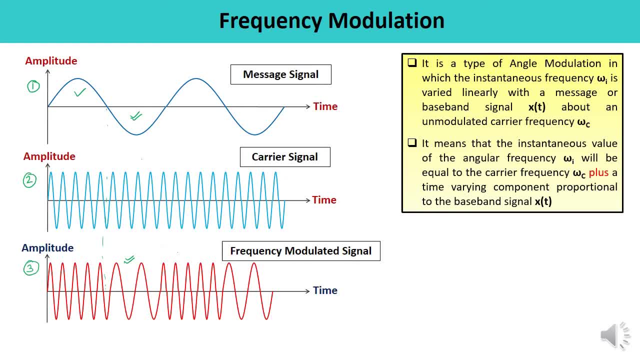 Where instantaneous frequency, which is denoted by omega i, it is varied linearly with a message or baseband signal about an unmodulated carrier frequency. The unmodulated carrier frequency is denoted by omega c, So this particular term can be expressed as omega i, which is the instantaneous frequency. 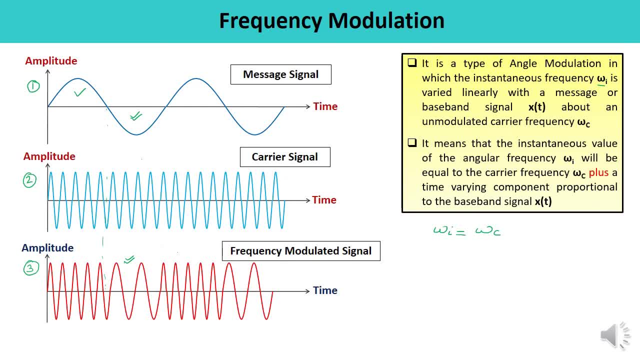 This is the sum of unmodulated carrier frequency Plus this particular message signal which varied linearly kf times, xt, And here this term kf. this is a proportionality constant and it is known as a frequency sensitivity. We will discuss in detail. 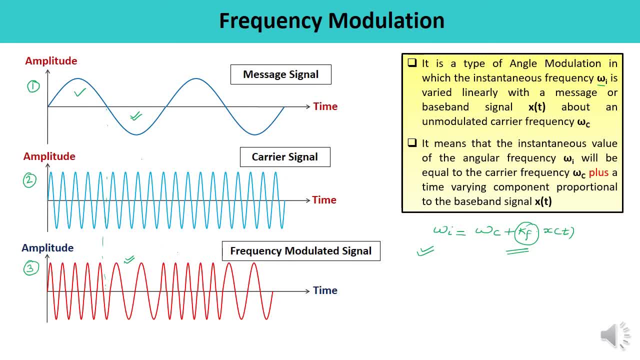 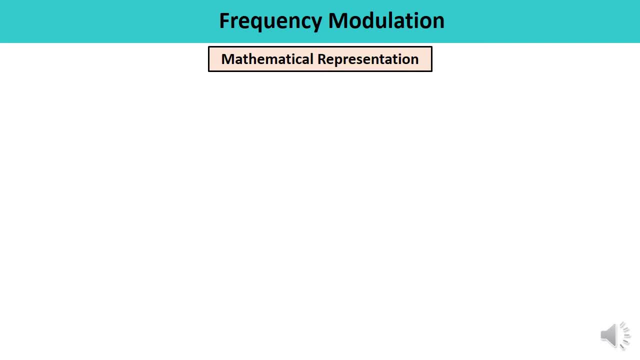 It means. this particular equation can be expressed in this manner. Let us derive a general expression for the frequency modulation. This is the frequency modulated wave. To start with, let us write the expression for unmodulated carrier signal. If the expression for unmodulated carrier signal is ct, it is equal to a cos, omega ct plus theta 0.. 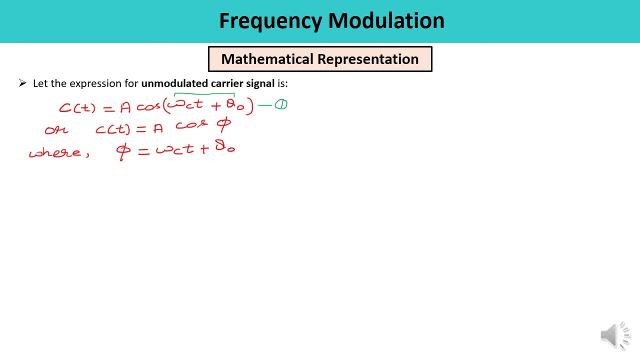 If we can write this particular term, omega ct plus theta 0 as phi, So this equation can be written as: what ct, which is equal to a cos phi, And here phi is the total phase angle of the unmodulated carrier. 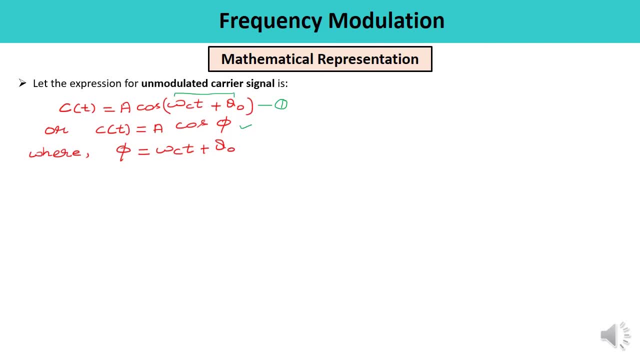 So if you have to write down the instantaneous phase angle, So instantaneous phase angle is denoted by phi i. So the equation of unmodulated carrier we can write as ct, which is equal to a cos phi, And in case of the frequency modulated amplitude remains same. 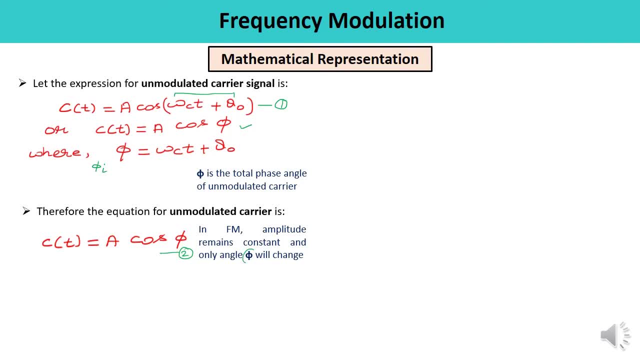 And only the angle phi will change, So this particular quantity is going to vary. over here It means now you can write down the expression of frequency modulated wave, which is denoted by st. That is what a cos phi i. 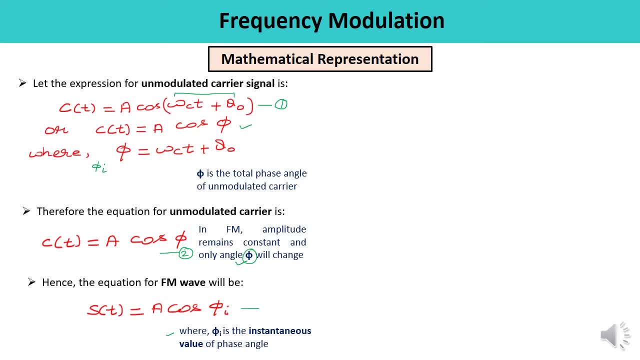 And phi i is the instantaneous value over here. So in this particular manner you can write down the equation of frequency modulated wave. Now to move on further. we know what is phi. That is omega ct plus theta 0.. 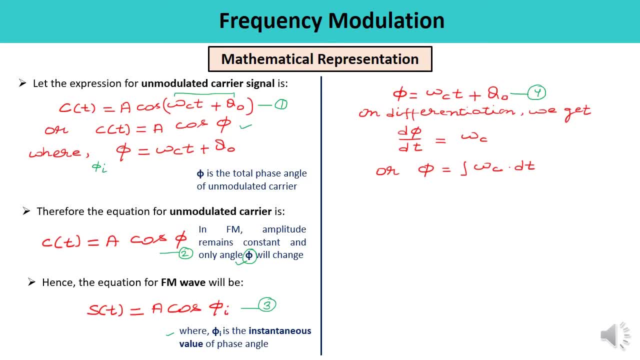 So we can differentiate this equation, equation number 4, with respect to the time. So what we will be getting, d, phi upon dt, which is equal to omega c, Or phi is equal to what Integral of omega c into dt. 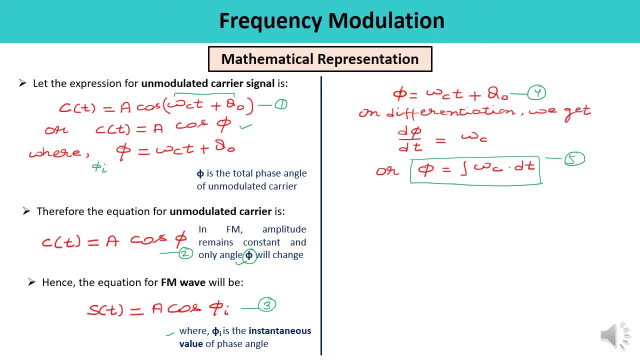 So this is what we are getting over here, Right? It means we can write down the expression for instantaneous phase angle, which is phi i. Phi i is what Integral of omega i into dt And what is omega i? Omega i is omega c plus kf into xt. 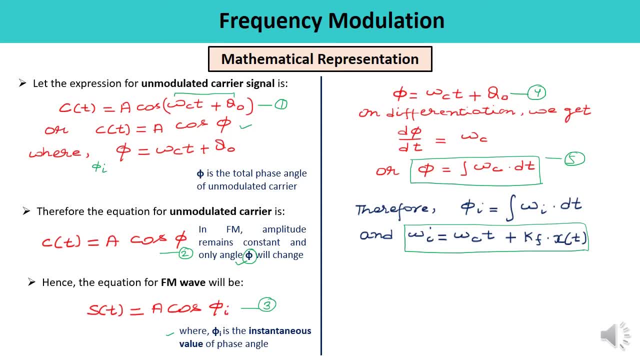 This is what we have discussed earlier. So now substitute this value of omega i integrated with respect to the time t, What you will be getting over here: Phi i, which is equal to omega ct plus kf integral of xt into dt. So this is what we are getting over here. 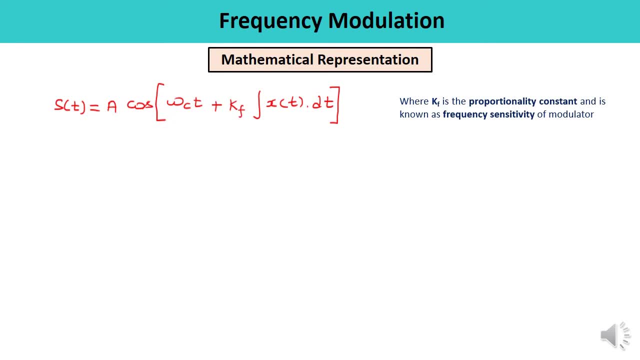 Moving on Here, kf is the proportionality constant and it is known as the frequency sensitivity of the modulator. This is a very important parameter. Now, in this particular integral, if we say phase angle of the unmodulated carrier, it is taken at t, it is equal to 0.. 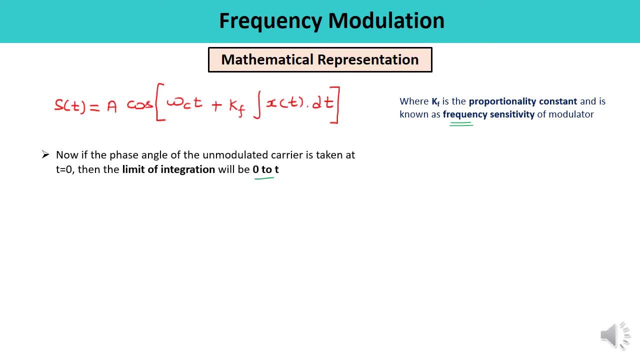 Then the limit of integration will be what It will be, from 0 to t. So now we can substitute the limits also 0 to t, So equation will be a cos, omega, ct plus kf, 0 to t, xt into dt. 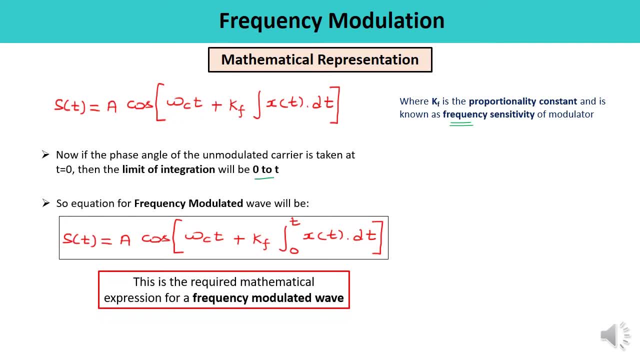 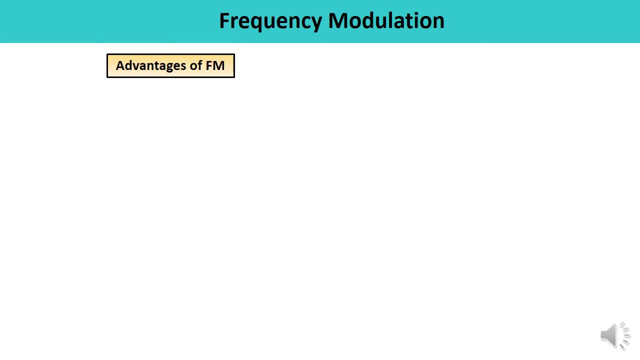 This is what the required general expression for the frequency modulated wave. Next, advantages of frequency modulation: Less interference. Noise is less over here. Power consumption is also less in comparison to the amplitude modulation. And in case of the frequency modulation the adjacent FM channels are separated by guard bands. 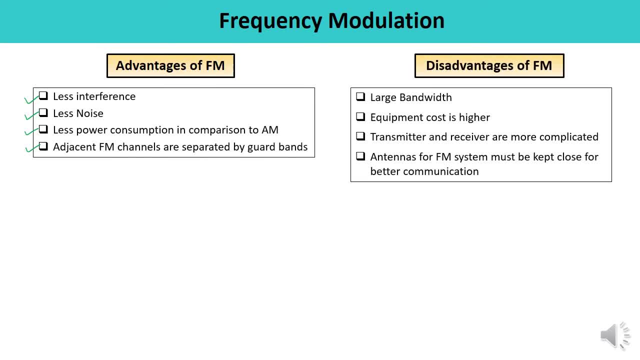 So these are the advantages. There are some disadvantages also. Large bandwidth Equipment cost is high, Even at the same time designing the equipment. this is also complex. Transmitter and receiver designing are more complicated And the very important point related to the antennas. 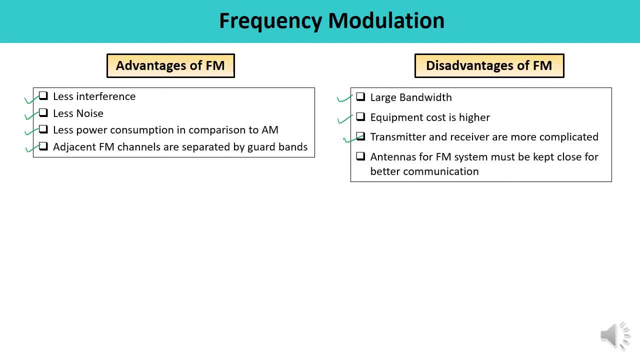 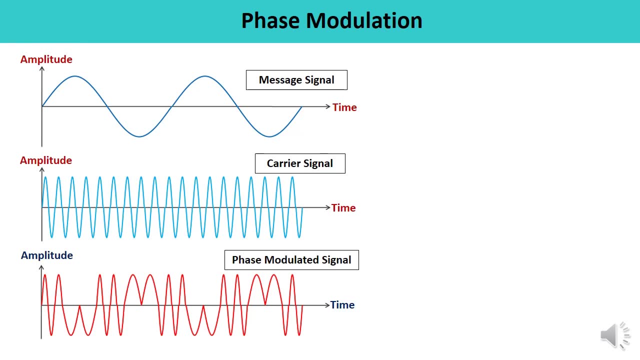 which are used for frequency modulation system, The antennas must be kept close for better communication. So these are the disadvantages for the frequency modulation. Next, let us discuss about the another type of angle modulation, which is the phase modulation. So in case of phase modulation, 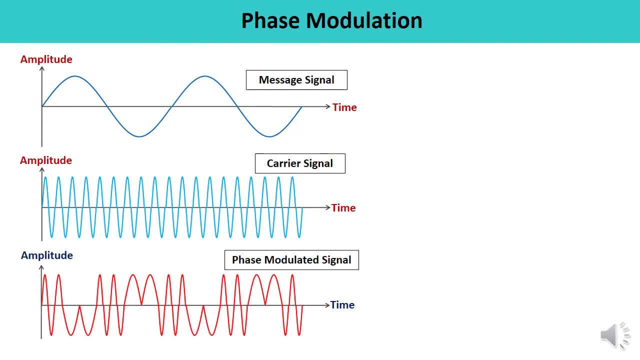 phase angle of carrier is varied according to the message signal. You can see one. This waveform is for the message signal. Second is the waveform for the carrier signal And you know that the phase angle of carrier is varied according to the message signal. 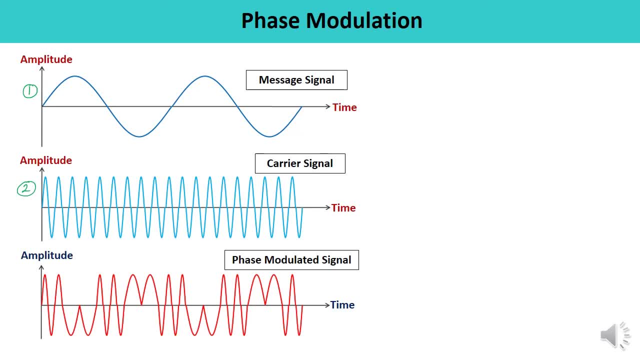 So you can see over here: When the message signal increases from zero to maximum value, the same carrier you are getting. But when this maximum value to the minimum value, you can see there is a change in phase Again while going from minimum to maximum value. 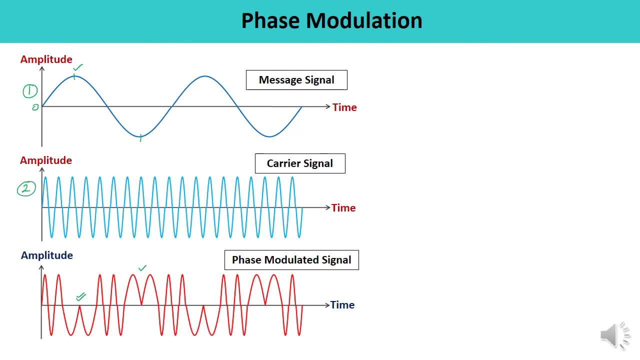 again, there is a change in phase. So you can understand this particular point, as the phase of the carrier is varying as per the message signal. So this is the case of the message signal, This is the case of the phase modulation, Or you can explain it as: 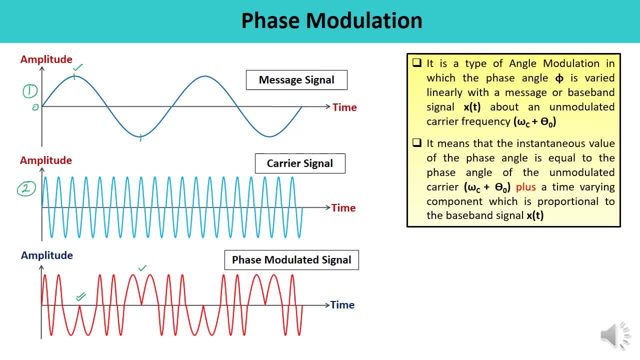 it is a type of angle modulation where phase angle, which is denoted by phi, it is varied linearly, with a message signal about an unmodulated carrier frequency. It means what If you need to calculate the instantaneous value of the phase angle? 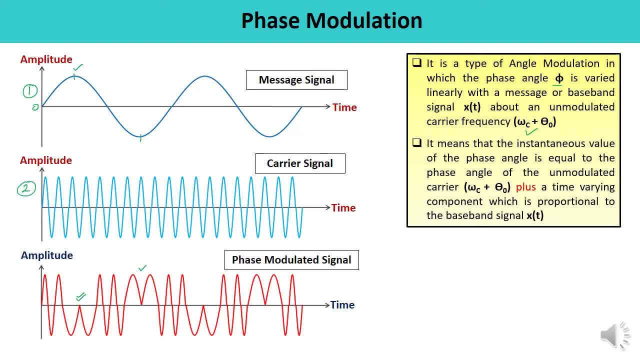 that would be equal to the phase angle of the unmodulated carrier, Plus a time varying component which is proportional to the baseband signal. It means what we can write over here. omega i, the instantaneous value. This is the sum of omega c plus a constant kp into xt. 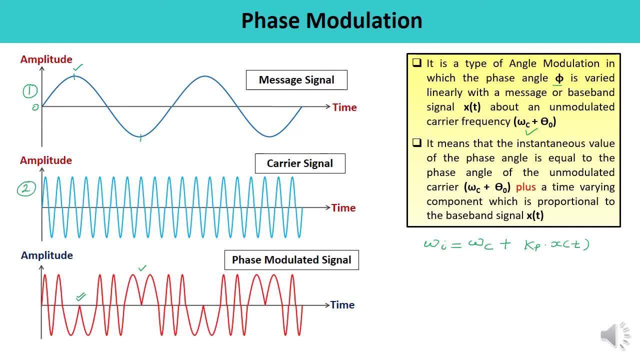 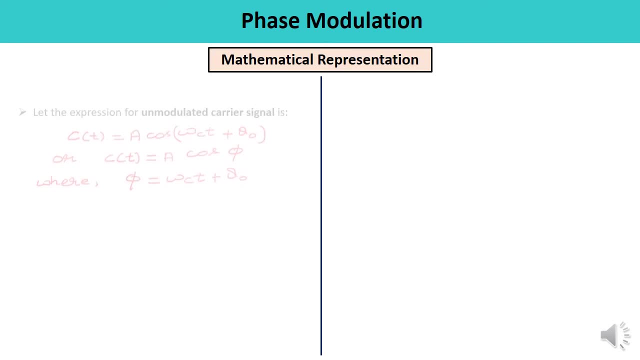 And here this particular constant, kp. this is known as a phase sensitivity of the modulator. Now let us talk about its mathematical representation. To start with, again, let the expression of the unmodulated carrier signal is written by this equation: ct is what? 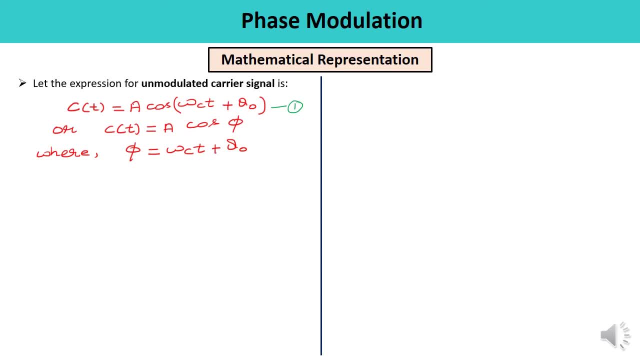 a cos omega ct plus theta naught. If omega ct plus theta naught is written as phi, so we can write it as what ct is equal to a cos phi. So here we are getting. phi is what omega ct plus theta naught. 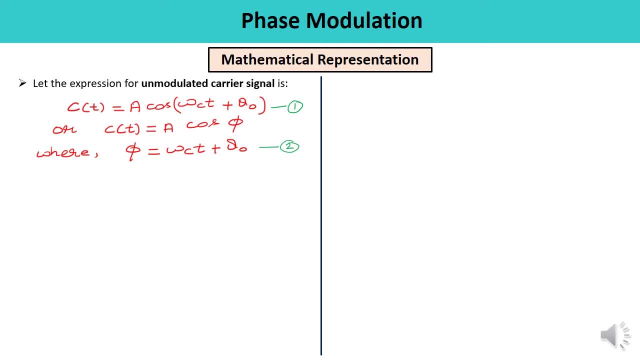 which we actually written for the simplification purpose. If, in this equation- number 2, we neglect this theta naught, If we neglect the value of theta naught, now the total phase angle of the unmodulated carrier would be written as what: 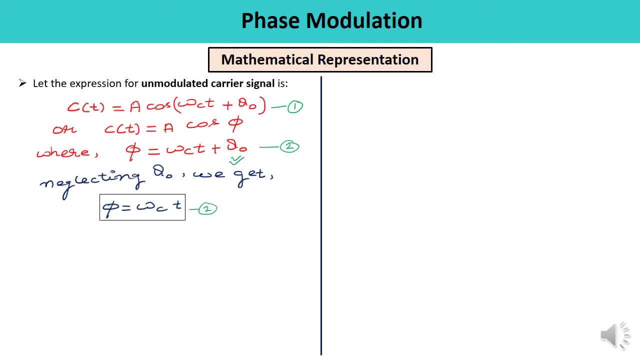 phi, which is equal to omega c into t. This is the total phase angle. Total phase angle of unmodulated carrier. Now, according to the phase modulation, you know that phase angle is varied linearly with a baseband or modulating signal. 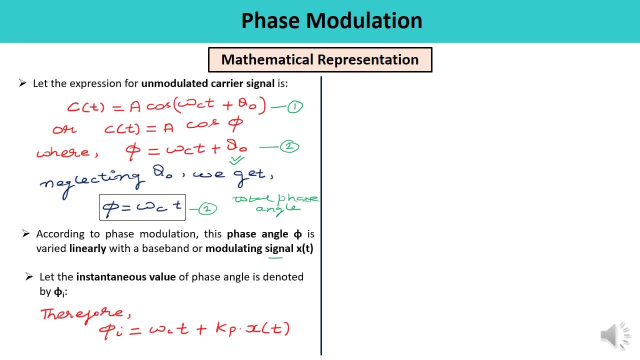 Now, if the instantaneous value of phase angle, if that is denoted by phi i, then we can write: phi i is what omega ct plus kp into xt. So in this particular manner we can write this equation. This is equation number 3.. 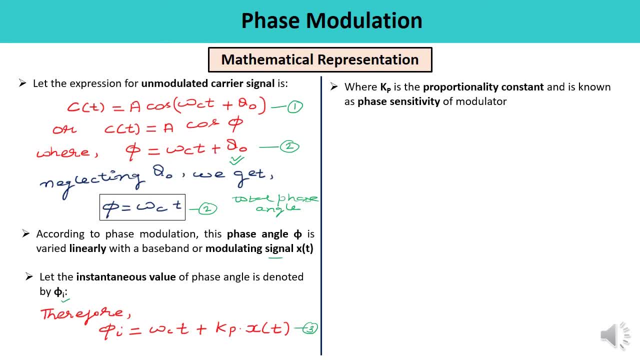 Now you must remember, and you must note it down, that kp is a proportionality constant. when we are talking about the phase modulation- And this is the phase sensitivity of the modulator- It means the expression for unmodulated carrier signal, what we have written over here. 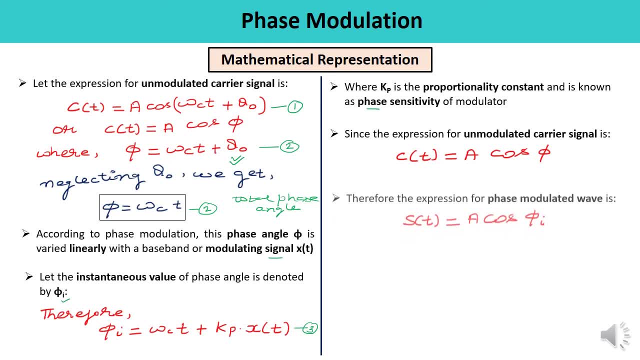 this is a cos phi, And here we can write down the expression for phase modulated signal. that is written by what? a cos phi i, which is represented by st. This is equation number 4.. Now here we can substitute the value of phi i. 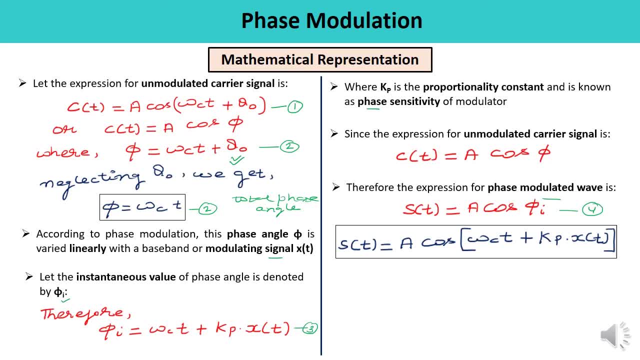 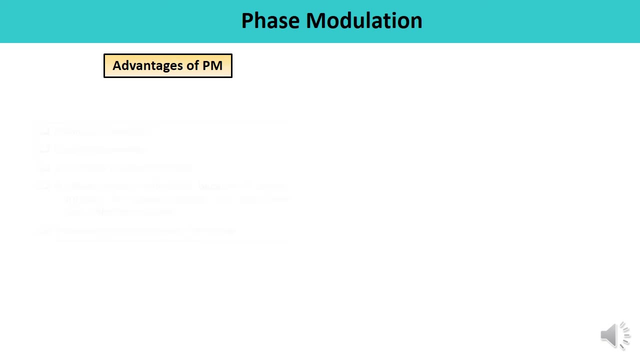 from equation number 3, which is omega ct plus kp times xt. So here we have substituted this particular value, and this is the required mathematical expression for the phase modulated wave. What are the advantages of the phase modulation? Phase modulation is simple to construct. 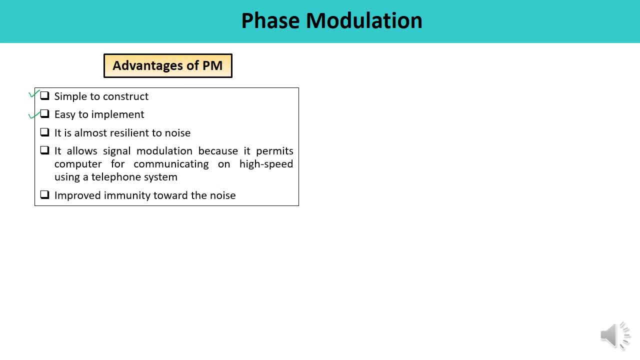 It is very easy to implement and it is almost resilient to noise. In this particular case, immunity is being improved towards the noise and it allows signal modulation. Because of this, it permits computer for communication on a very high speed using a telephone system. 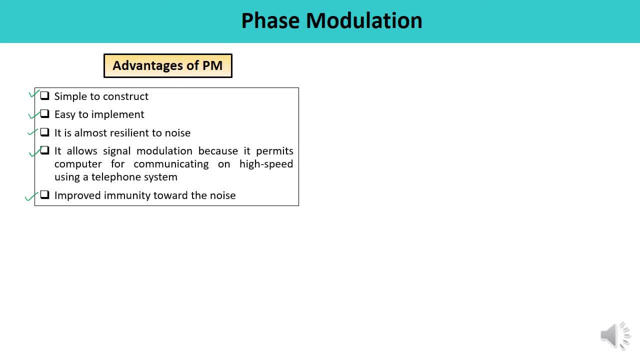 So these are the various advantages of the phase modulation. Now disadvantages: It requires two signal and there must be a phase difference between them. It requires more hardware equipment to construct. because of its conversion approaches, Phase ambiguity also arrives if the modulation index exceeds to 180 degree. 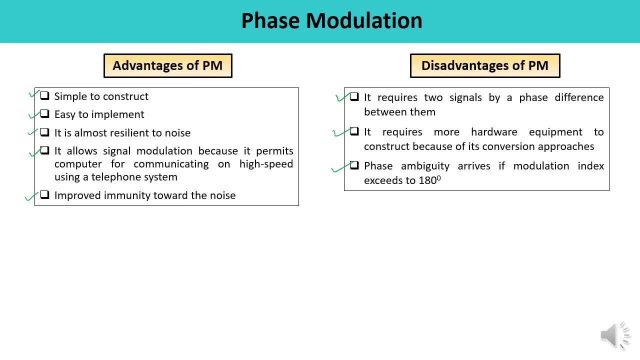 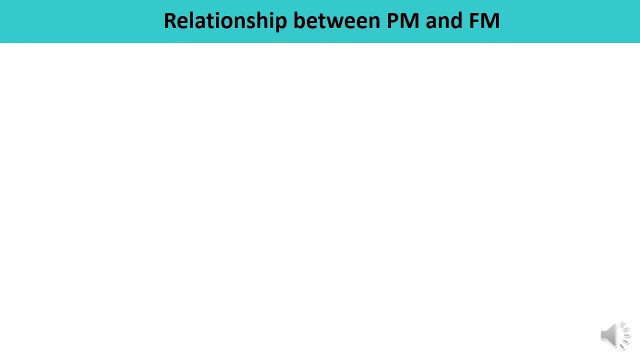 So there are various disadvantages also of phase modulation. Now let us talk about what is the relationship between the phase modulation and the frequency modulation. Till now we have derived a general expression for frequency modulated wave. We have derived a mathematical equation. 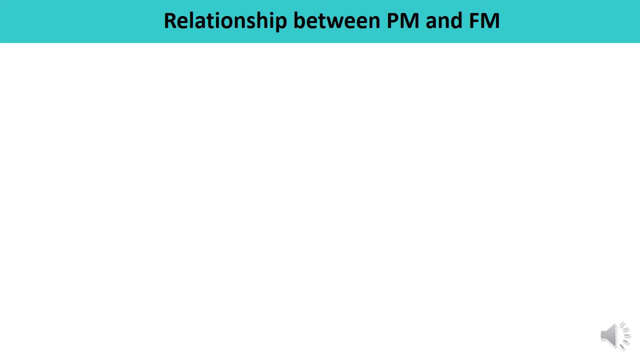 for the phase modulation wave. But what is the relationship in between these two, Frequency modulation and phase modulation? they are closely related to each other because in both of the cases there is a variation of total phase angle, because both are the types of angle modulation. 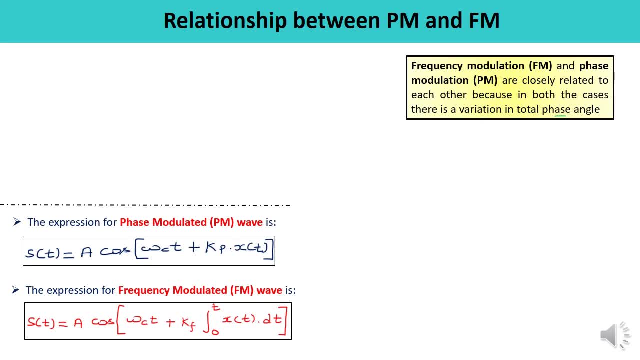 These are the equations which we have written for the phase modulation and the frequency modulation And you can observe from these equations that phase modulation and frequency modulation, they are closely related. And if you observe this equation number, this equation number 1, which is about the phase modulation, 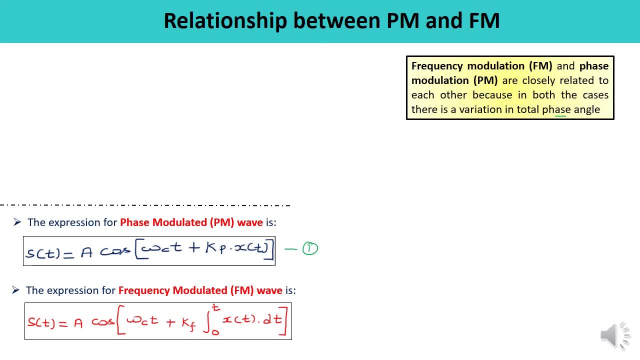 here, phase angle varies linearly with the message signal, which is Xt, Whereas in case of the frequency modulation, which you have written by using equation number 2, the phase angle varies linearly with the integral of the message signal or the baseband signal. 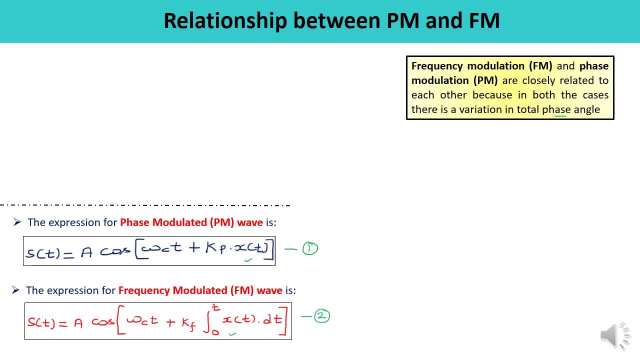 It means frequency modulated wave. FM wave can be obtained by using PM, and vice versa is also true. Let us see. You can see a diagram which is being shown for the generation of FM using phase modulator, So to get an FM signal. 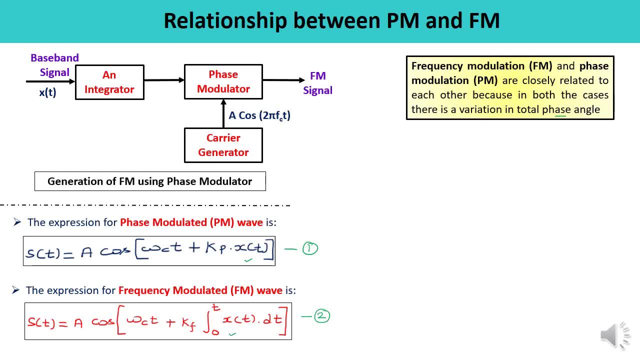 by using phase modulate, by using PM. you can see, first we integrate the baseband signal- Here our integrator is being shown- and then this particular signal is applied to the phase modulator Right. So this process, the overall process, is being 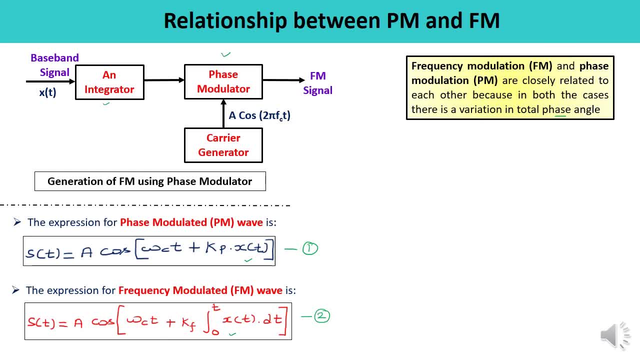 like, explained with the help of this block diagram and at the output what we are getting. we are getting the FM signal. Same is the case with the generation of PM phase modulation using the frequency modulation. So here, PM wave may be generated by using frequency modulator. 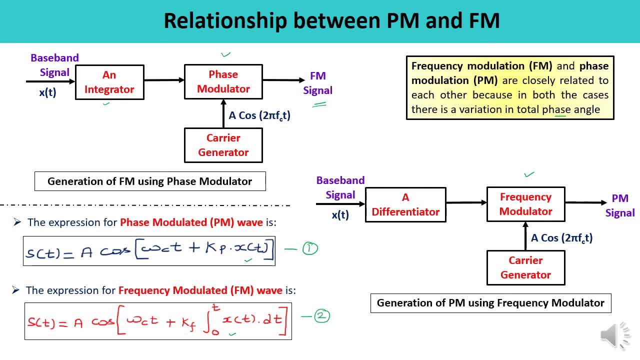 You can see the frequency modulator over here by. but first the signal must be differentiated. You need to differentiate the baseband signal or the modulating signal and then apply it to the frequency modulator So the overall process can be performed. and at the output.